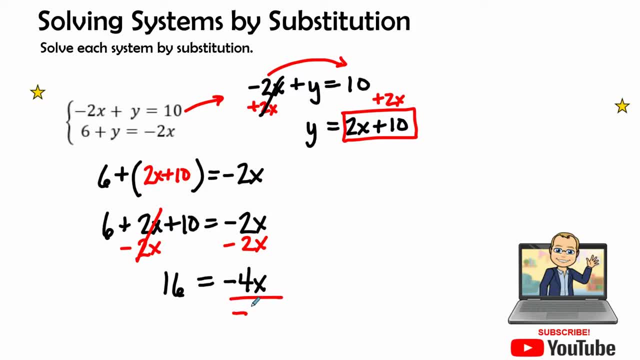 So I'm going to divide the negative 4x by a negative 4 on both sides, which gives me an answer of x, And this is a positive 16, divided by a negative 4 is a negative 4.. So I can flip that around. so my answer is: x equals a negative 4.. 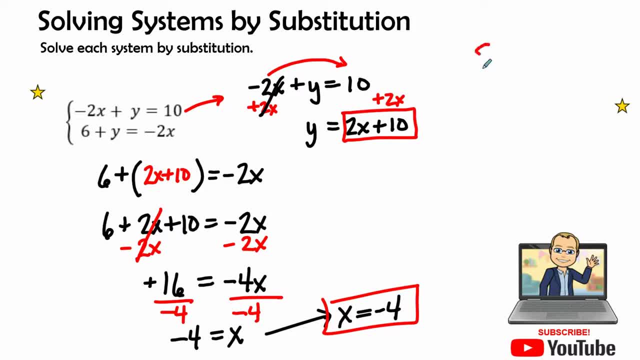 So this is my x value in the solution. And now I have to go ahead and find my y value. And to find my y value I said box to box, So I'm going to plug in A negative 4, wherever I see an x. 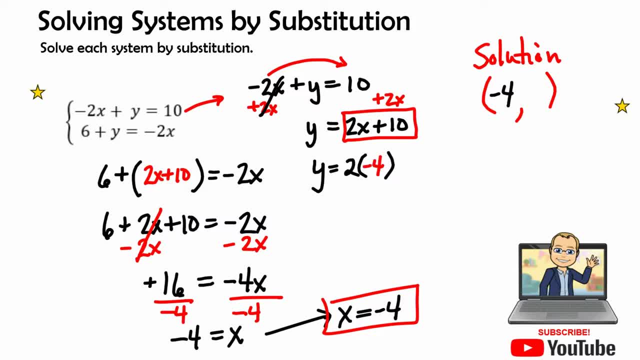 And so right there, by that 2x I'm going to plug in that negative 4, and then write the rest of the equation. y equals 2 times a negative, 4 is a negative 8, plus 10.. That combined like terms, and so the y equals a positive 2.. 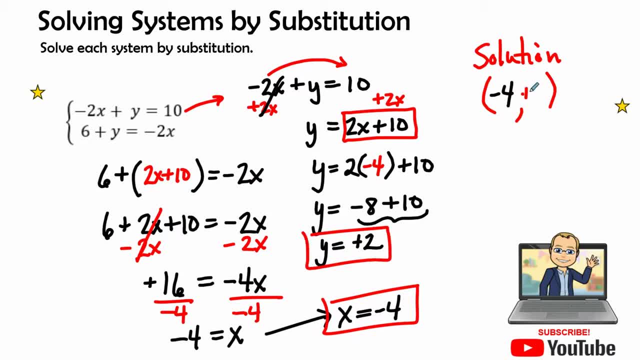 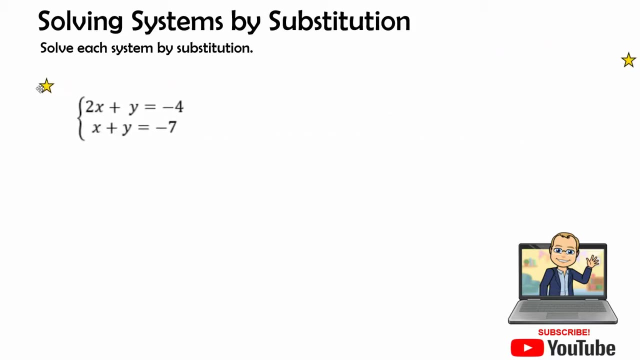 There is my y value. So in this equation of this system, I know that my solution is a negative: 4 plus 2.. Let's go ahead and try another equation. Let's go ahead and move this one back And my next one that I'm going to pull out here. 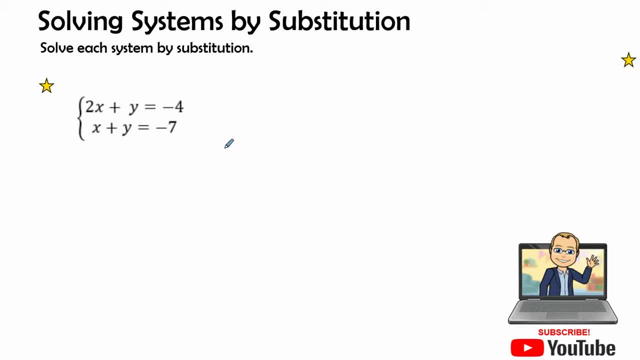 I can look and see what can I isolate really easy. Let's try the bottom equation this time. So I have x and x is negative 4.. So I have x plus y equals a negative 7, where I see that this x can be moved over by adding a negative x to both sides. 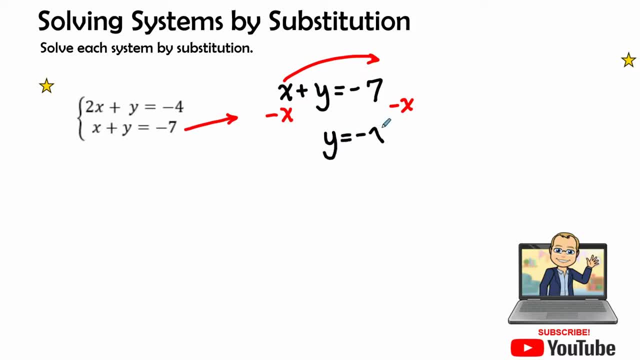 So now I have: y equals a negative x minus 7.. Remember, x minus x cancels each other out or creates a 0. And I know that this expression of negative x minus 7 is going to be plugged into now. our first, our top equation. 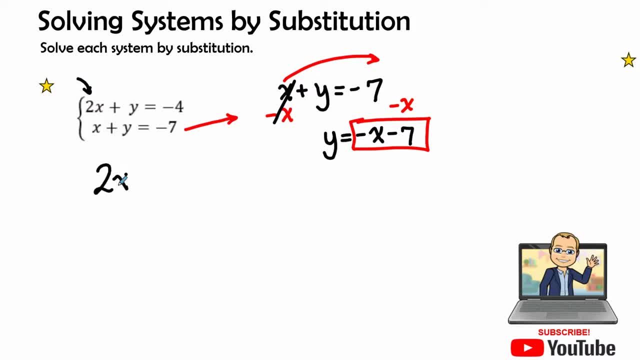 We're going to go ahead and write our top equation of 2x plus y And the y we're going to substitute this expression in for y, So I'm going to open up my parentheses. Equals a negative 4.. So when I substitute in this negative x minus 7..